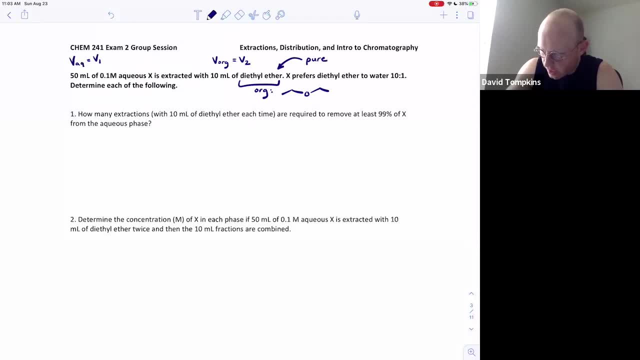 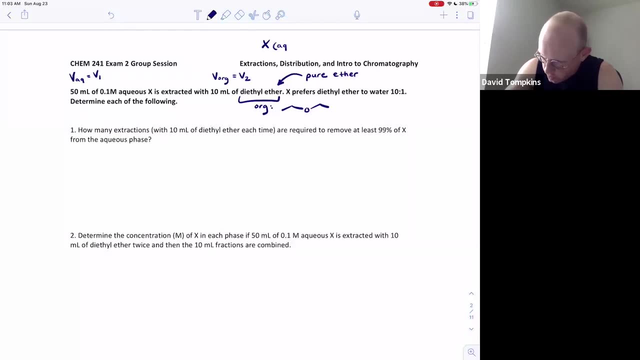 this ether is pure, It's not containing any X, And X is going to reach some equilibrium where it originates in the aqueous layer. some of that exits and enters the organic layer and we get some k-part or equilibrium constant And that k-part value or the concentration of X in the organic layer. 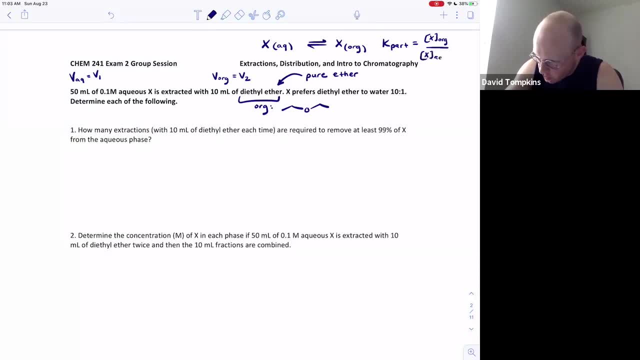 relative to the concentration of X in the aqueous layer, we're told is 10 to 1, or prefers diethyl ether to water, 10 to 1, right, Which means that X is probably quite non-polar, since it prefers to be solvated in the non-polar. 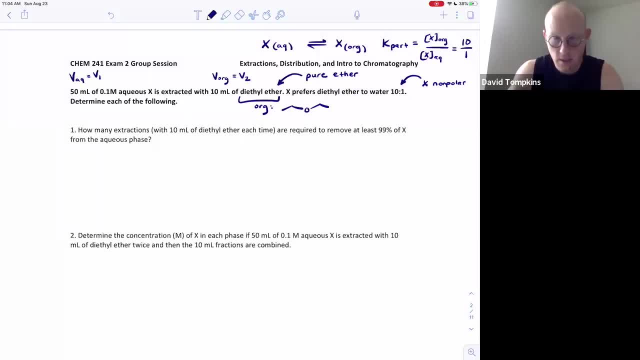 organic diethyl ether phase. First question here: How many extractions with 10 mils of diethyl ether each time? So we're looking for N. How many are required to remove at least 99% of X from the aqueous phase? So recall that. 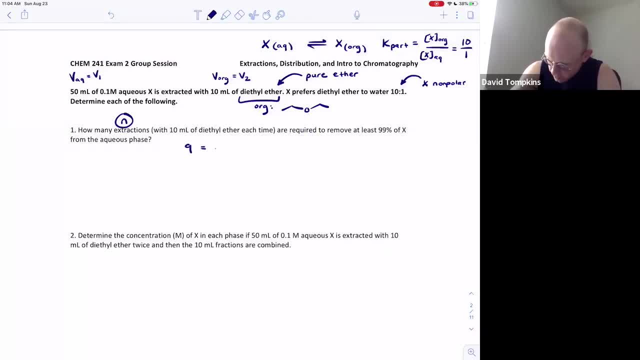 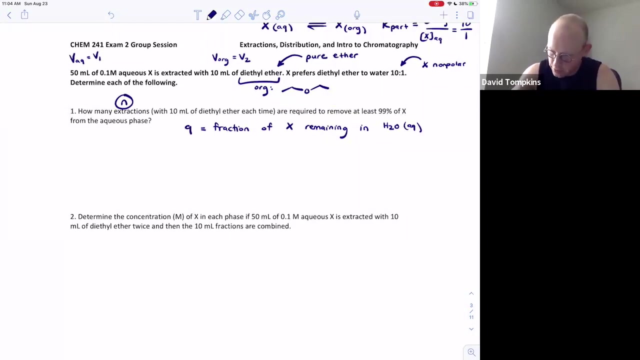 Q is the fraction of the solute X that remains in the original phase, or the water. So we want to remove Right, At least 99%, Or we want Q to be less than or equal to 1% right, In other words, in terms of a. 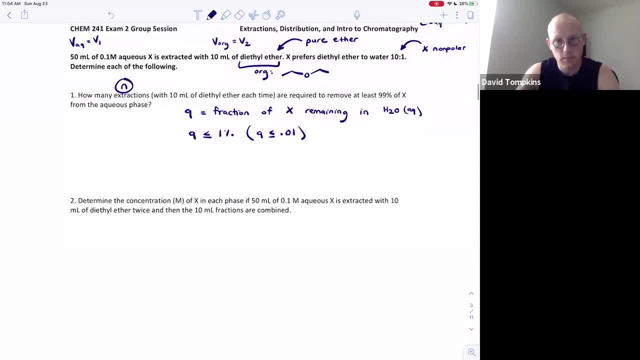 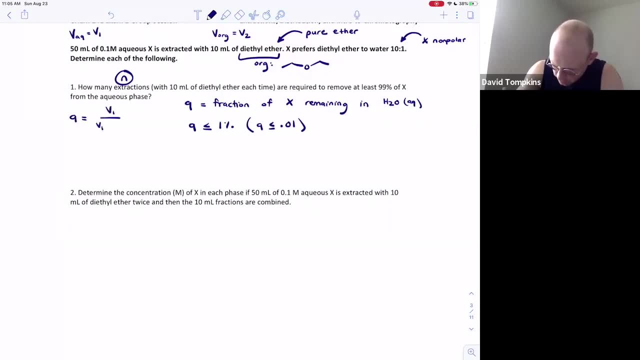 fraction, it's less than or equal to 0.01.. So we can set up our Q equation here right. Q is equal to volume 1 over volume 2, plus the partition coefficient multiplied by volume 2, all raised to the N number of extractions. 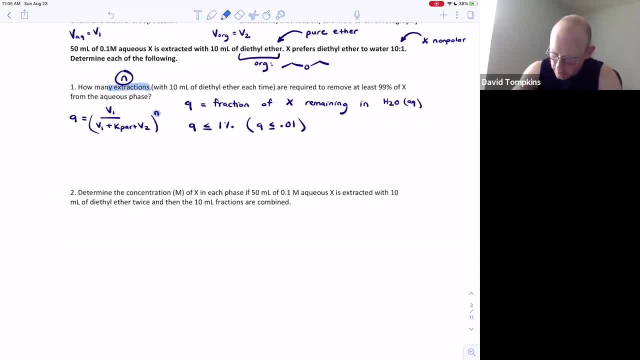 And we are searching for this N number of extractions here. So Q the largest it can be is 0.01.. And the volume 1 is 50 mils of the aqueous solution. Over that same volume I'm excluding the. 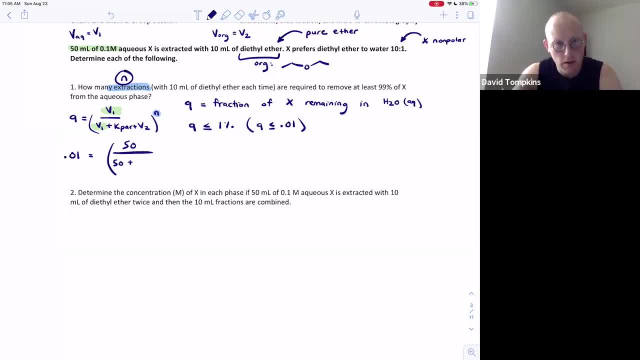 units, because as long as we use the same volume unit milliliters, this is just the unit. Let's see if we can find out how much we can get out of this fraction plus the partition coefficient times the volume, volume 2.. 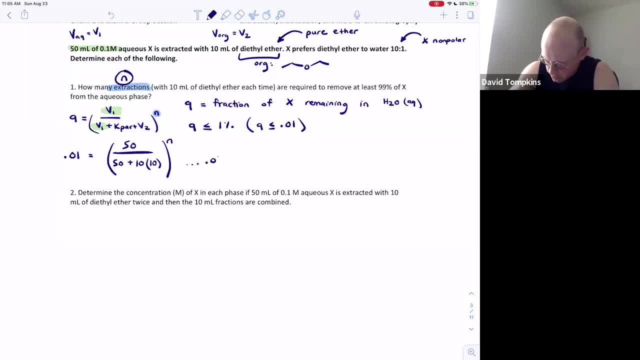 So if you want to solve this right, we can now say: 0.01 equals 50 over 150, or is equal to one third raised to the N. And to solve for this exponent N we need to take the log of each. 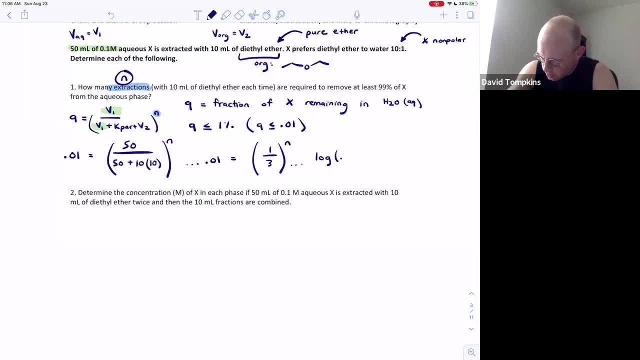 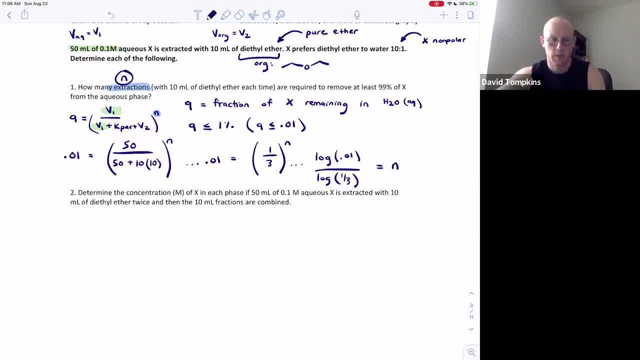 equal to N. So I took the log of each side and then isolated N for N. you should get 4.2. And 4.2 indicates that you do four extractions and then 20% of a fifth extraction. But this is not. 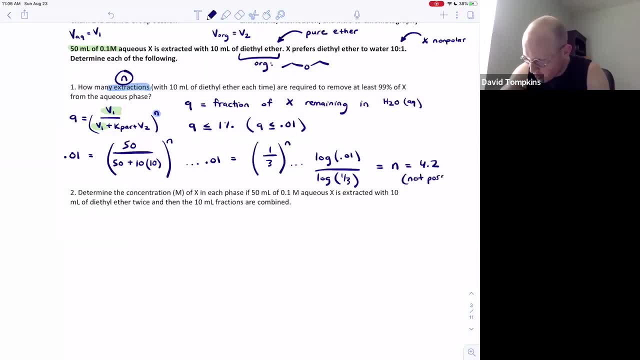 possible, But this is not possible, But this is not possible. Our limitations are that we are working with team portions of diethyl ether, So we either do the diethyl ether extraction four times or we do it five times, And if you want to get at least 99% out, we are going to round in up. 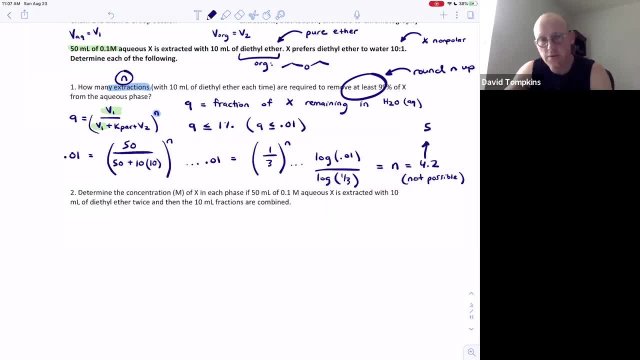 And if you want to get at least 99% out, we are going to round in up: Or the only reasonable number of extraction to do to ensure that we will remove at least 99.5 percent N, Or the only reasonable number of extraction to do to ensure that we will remove at least 99.5 percent N. 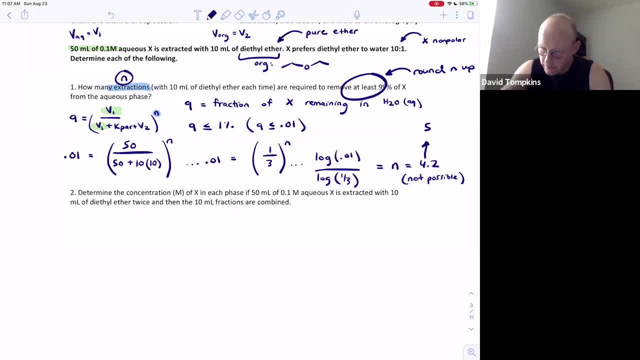 other 노력 code percent is five full extractions, Or the total volume of the ether. the organic layer would be 10 mils times five. We would do 50 mils total consumption of ether. So the next problem: we're determining the concentration of X in. 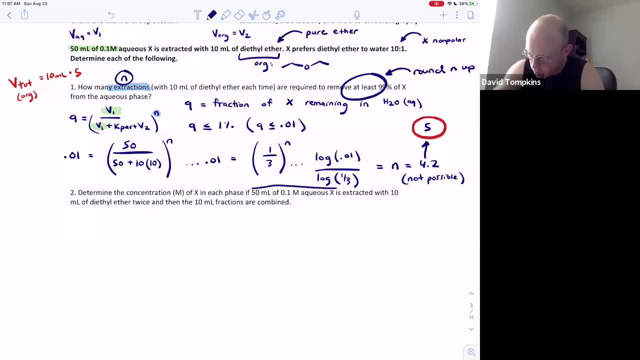 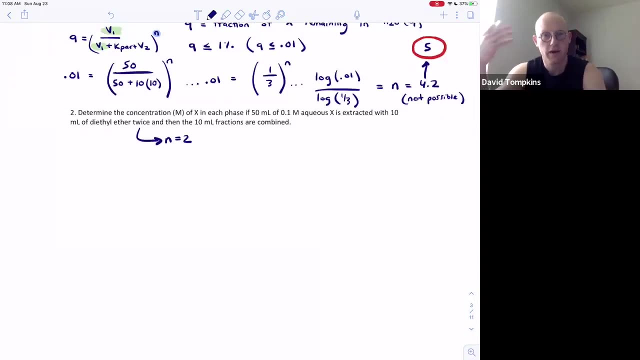 each phase. after that, same 50 mil 0.1 molar aqueous solution is extracted with 10 mils of ether twice. So we do two extractions, or n equals two. So to find the molarity in each phase we need first to find the volume in each phase. 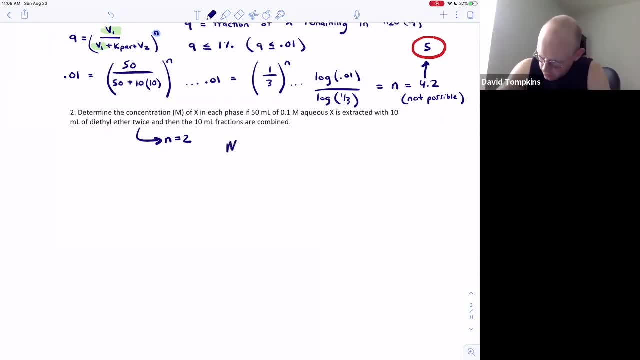 And then of course you can say the molarity of X in the aqueous phase would be the moles of X divided by the volume aqueous, And that volume is 0.05 liters. Alright, we have 50 mils. The molarity of X in the organic phase. 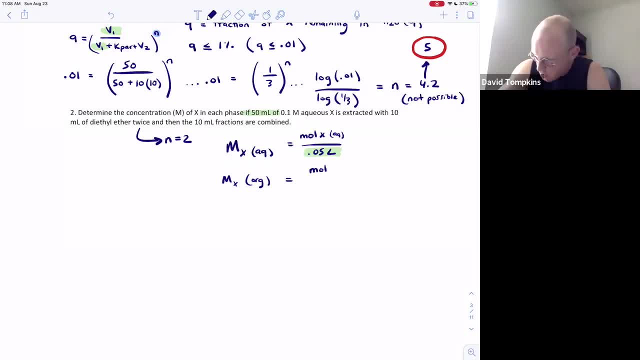 is going to be $2 bri. The organic phase is $1.5 bri. So then when we put all of the molees into one cap, that means they're going to have zero consents. So that makes $2 bri to be the moles of x that have partitioned into the organic phase, divided by the volume of the 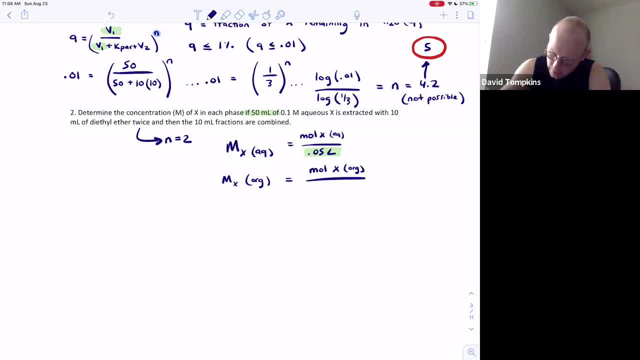 organic. It says we use diether right twice, that's the organic layer, 10 mil fractions at a time, and then we combine them. So this is going to be 0.01 liters first time and then we're going. 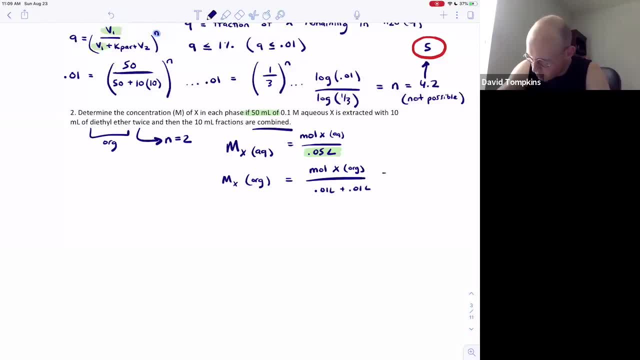 to combine it with the other 0.01 liter or 10 mil fraction. So the final molarity of x in the organic phase is going to be the moles of x in the organic phase over 0.02 liters. Okay, so now we just need to find the moles of x in each phase, which means first use the fraction. 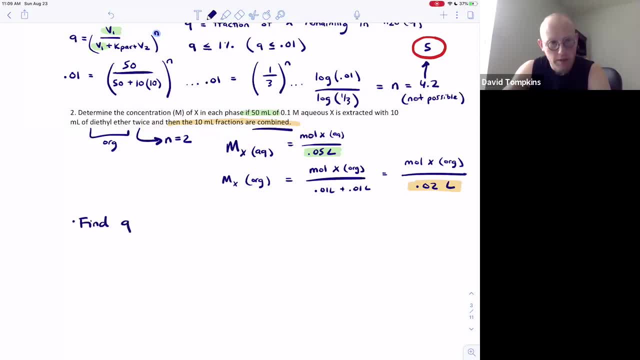 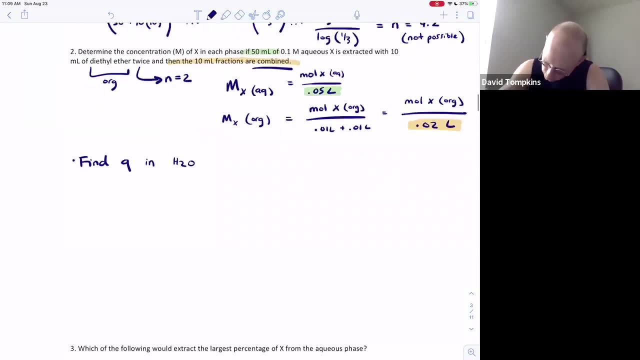 equation Five, the fraction of x, q right that remains in the water. So q is equal to the volume of water over the volume of water, plus k, part times the volume of the ether raised to the n, or this is equal to 50. 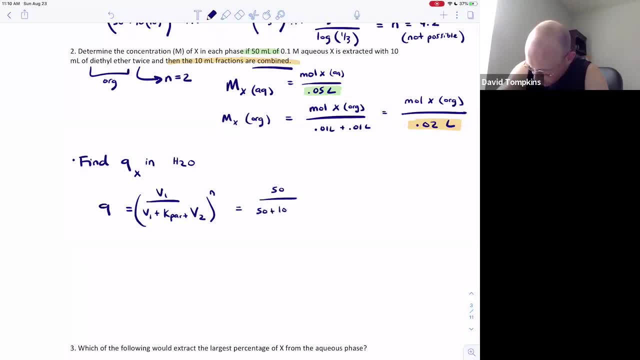 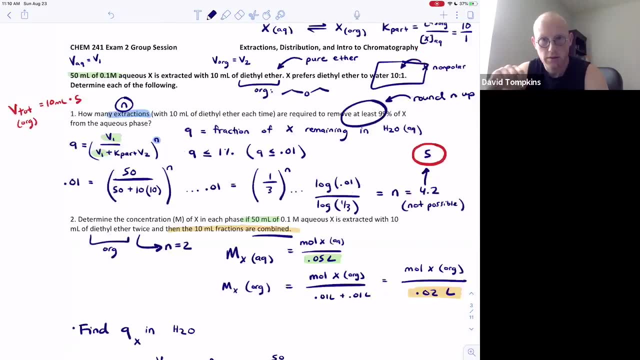 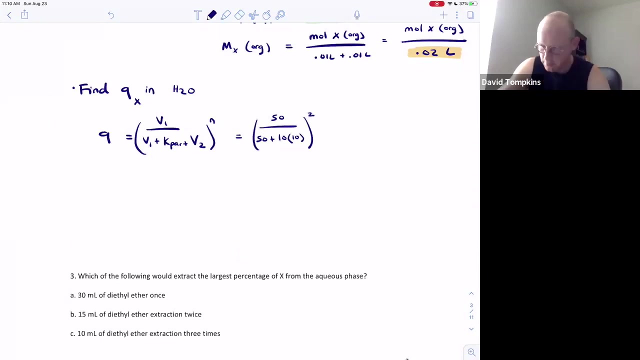 over 50 plus 10.. So k part was 10, we saw that We were given that value up here where it preferred ether to water, 10 to 1.. And we're doing 10 mil extractions two times. So if you solve for this, you'll see that it's. 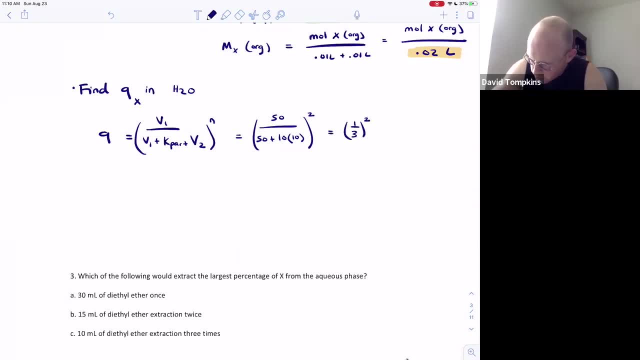 1-ninth is one-third raised to the two power, or one-ninths, Okay, which means that 1 minus q right, or the fraction of x that is going to the organic phase, the ether, is 1 minus one-ninth or 8-ninths. 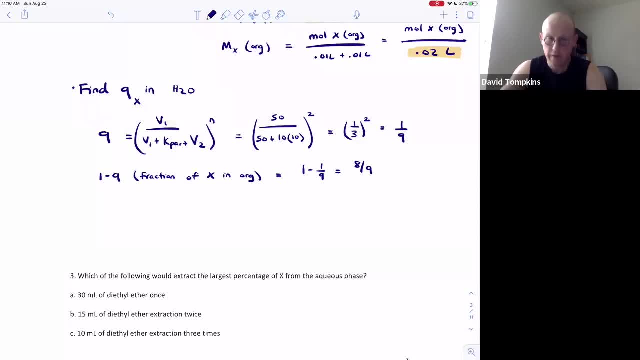 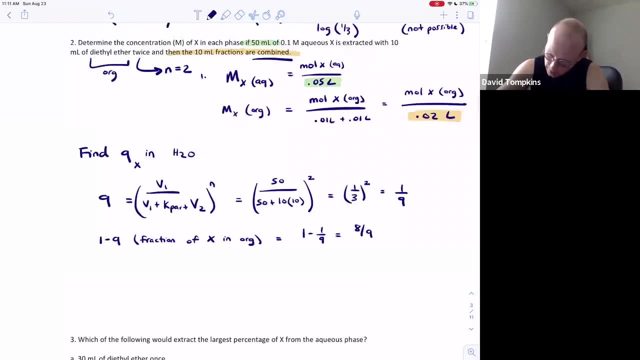 Okay, well, let's go back and look at the fluidity and how we can work this. So now we know the fraction of X at each phase. That was step one, Or I guess we can say: writing molarity equation, step one. 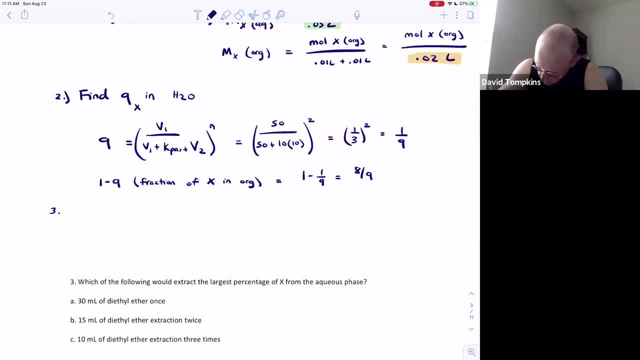 finding the fraction. step two. Now, if we can just figure out what the total moles of X were in the beginning, we know that one ninth of those total moles are now staying in the aqueous layer And the other eight ninths have gone. 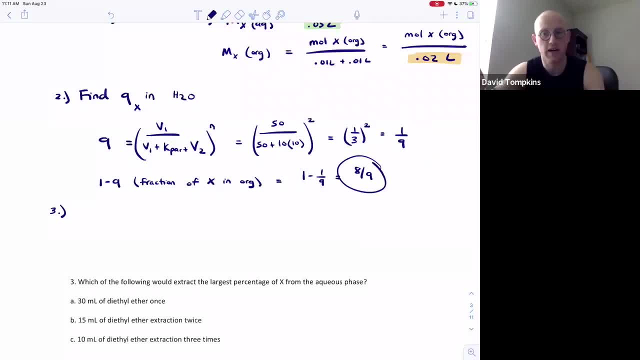 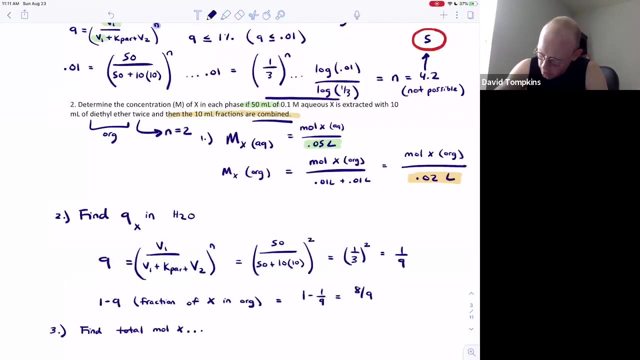 into the organic layer. So if we just know the total moles, we can use the fraction to find the actual moles in each layer. So the total moles of X. X originated only as an aqueous solute. It was 50 mils 0.1 molar. 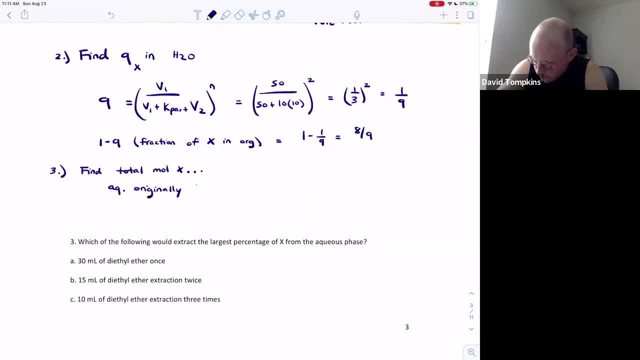 Because it only originally was in the aqueous phase. I can use the molarity. It was 0.1 moles of X per one liter of water And we have 50 milliliters of water or 0.05 liters. 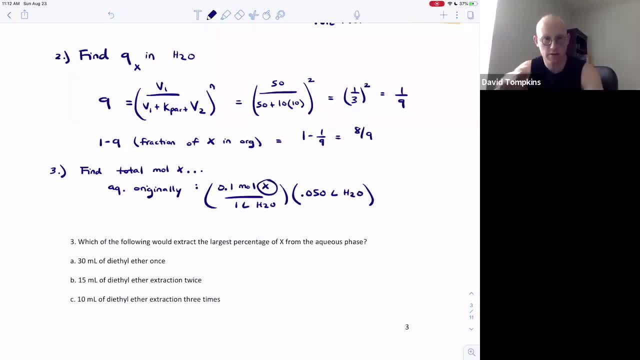 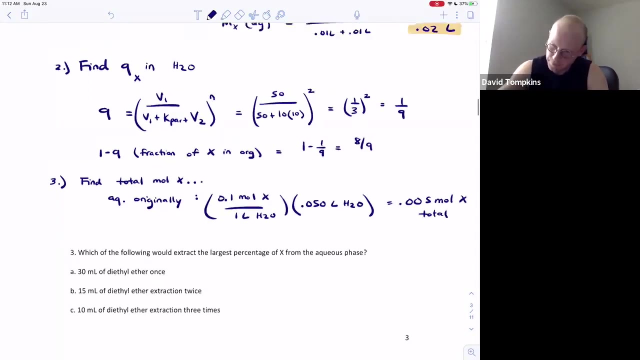 So only use the volume containing X originally, Don't use the other volume of the pure solvent. So 0.1 times 0.05 is a total of 0.005 moles of X. So from here we can now find the moles of X in each phase. 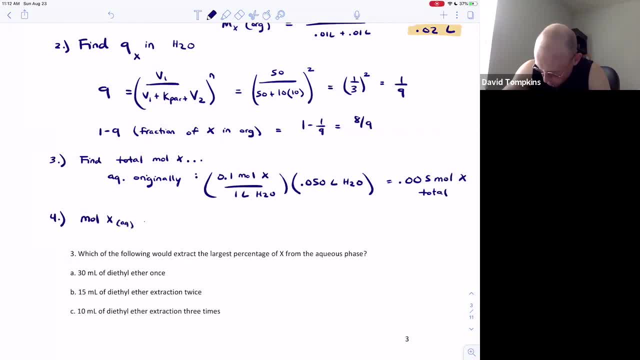 So the moles of X in the aqueous layer will equal the one ninth, because one ninth of the moles remain times 0.005.. And the moles of X in the organic layer is eight ninths times 0.005.. 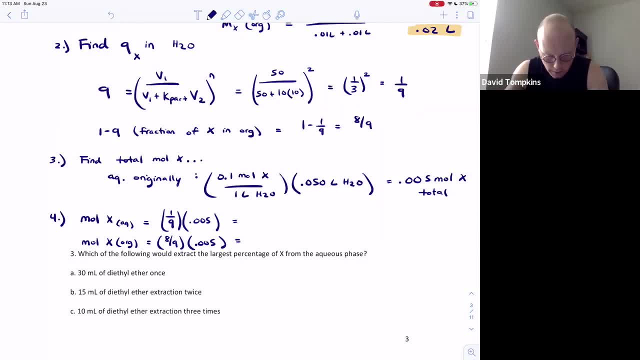 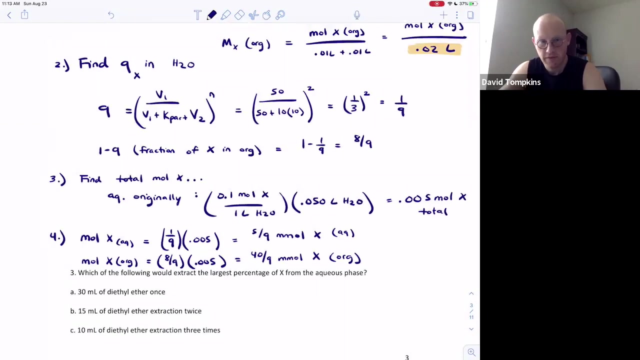 So if you calculate those values, you're going to get essentially five ninths of the moles of X in the aqueous and 40 over nine milliboles of X in the organic. And finally step five, plugging back into the molarity equations. 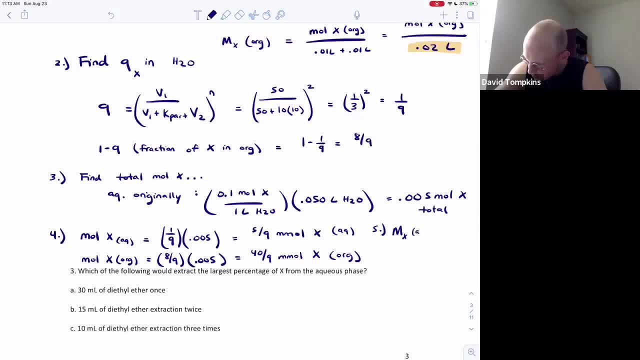 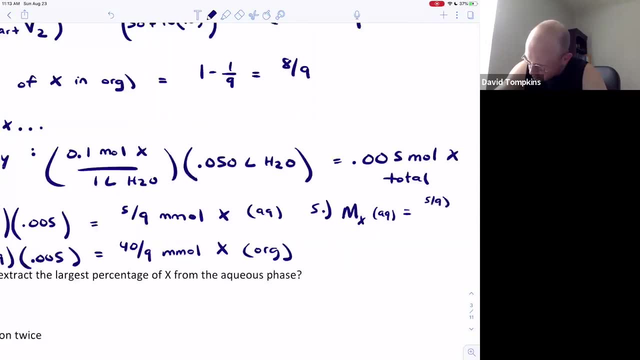 the molarity of X in the aqueous layer will equal the millimoles, So that's 0.005 over the milliliters 50. Millimoles per milliliter gives moles per liter because the milli cancels. 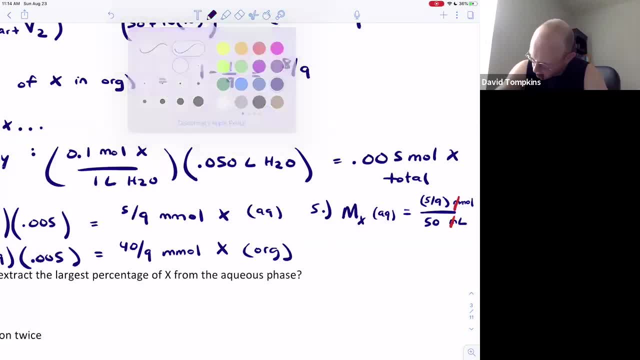 And the molarity of X in the organic layer is the other mole value. we found 40 ninths over 20 milliliters because we combined the two 10-mil fractions. Once again, milli cancels out to give moles per liter. 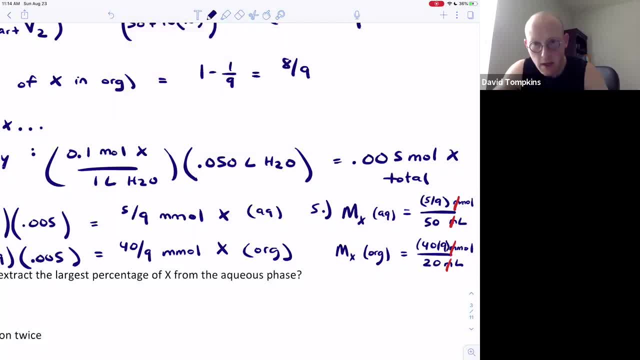 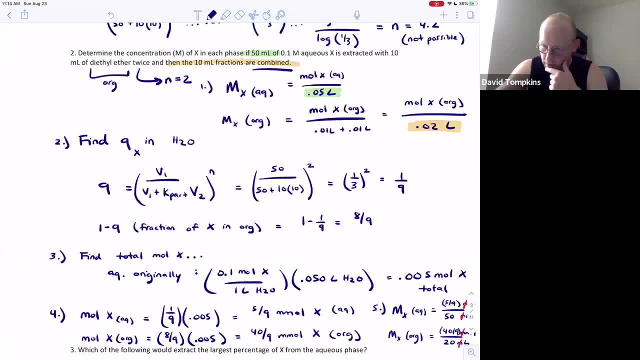 So you can solve those out explicitly and you'll get some decimal values. So, overall, if you're given an original concentration of some solute and then you do an extraction, these steps are those that you follow to find the final concentration in each phase. 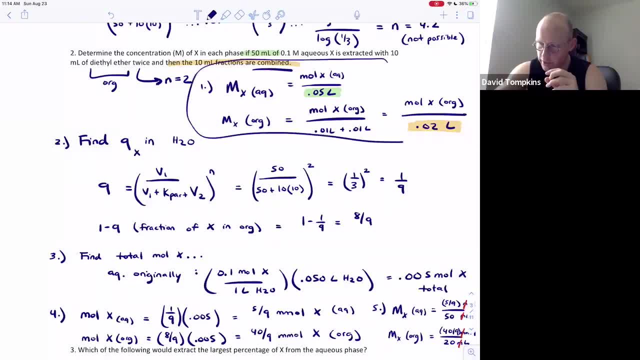 after n. number of extractions. right, We first write the molarity equations. It's just moles of X divided by the volume: 1, 0, 0, 0.. volume of that phase, and then we find the fraction that remains in the original phase. 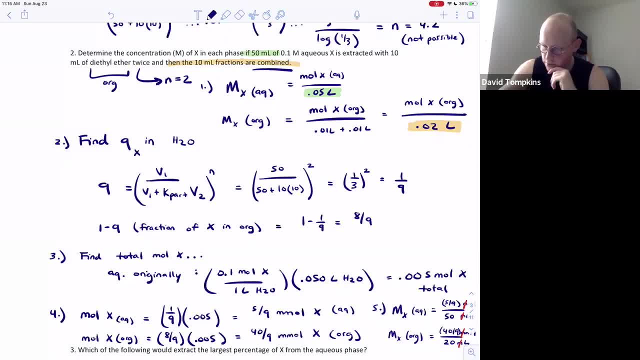 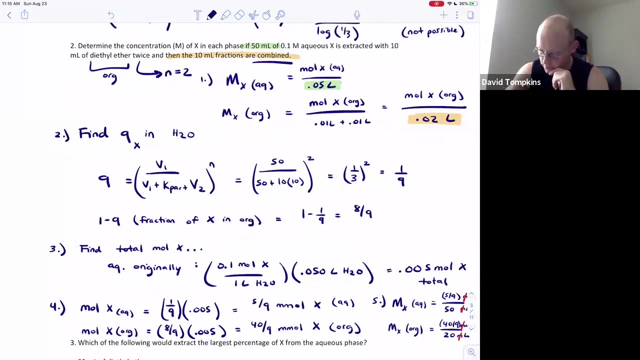 after n-number, or in this case, two extractions. with 10 mils of diethyl ether, We found that to be one-ninth remains and eight-ninths partition into the organic phase. Next, you simply find the total moles of x and then multiply the fraction of each phase.